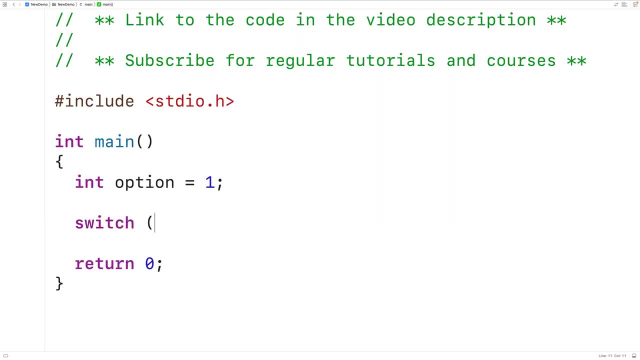 Then here we'll make a switch statement with the expression option. Then we'll have a couple cases. We'll have case 1 and then case 2.. And for case 1 we can just output option 1 selected. So we'll have option 1 selected, followed by a new line. Then in here we could have an if statement. 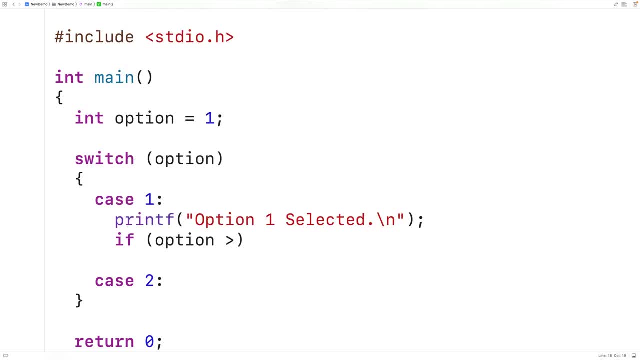 So we could have here if option is greater than or equal to 1.. And then we could have the body of the if statement. Now case 2 here can actually go inside the body of this statement. This is valid And we could have statements underneath case 2.. We could have here printf: option 2 selected. 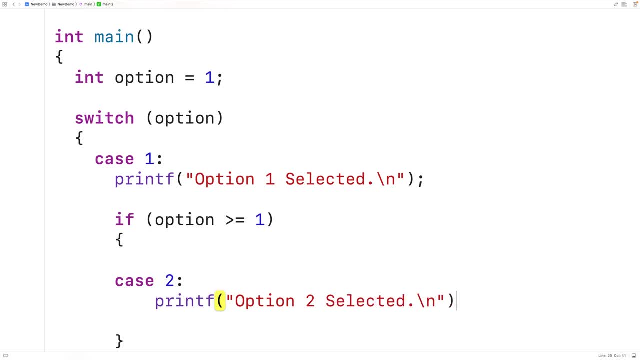 followed by a new line. Now, if we save, compile and run the program now, we're going to get option 1 selected, followed by option 2 selected, because there is no break after printing out option 1 here. The if statement body will execute and we're going to output option 2 selected. 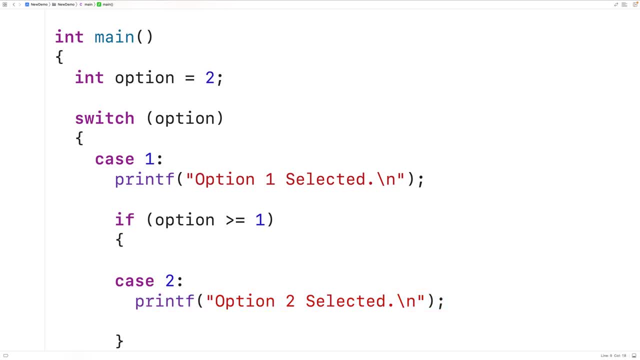 But if we change option to 2 here and then save, compile and run the program now, we get option 2 selected. So even though this case is in the middle of this, if statement body, this is going to work. This is actually a thing that you can do with switch. 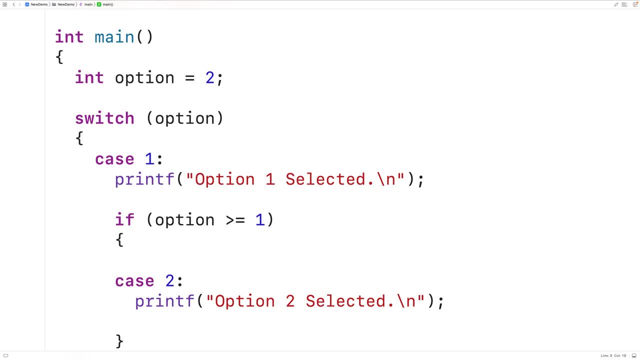 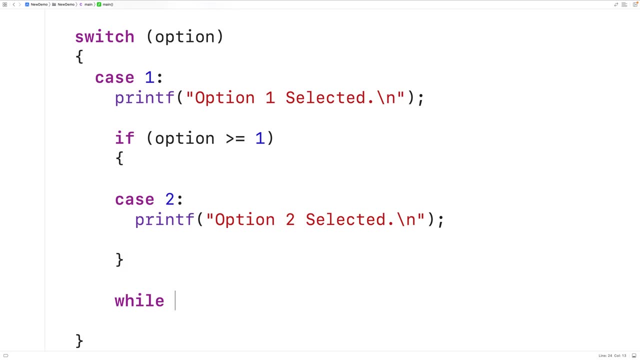 statements and other control structures in C. We can also do this with loops. So for example, underneath case 2 here we could have a while loop. We could say: while option is less than or equal to 10. Then we'll have inside this while loop option plus plus to increment option with each loop. 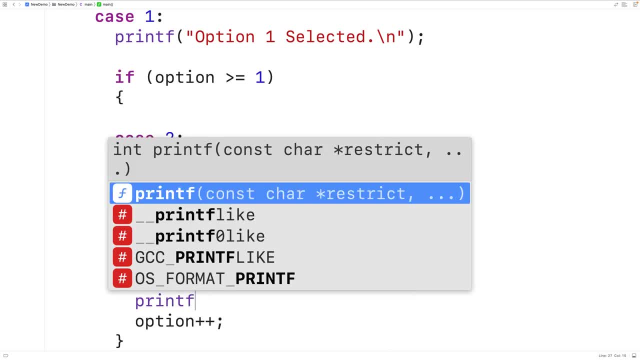 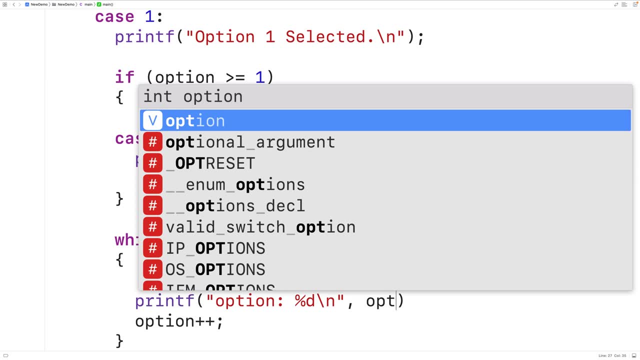 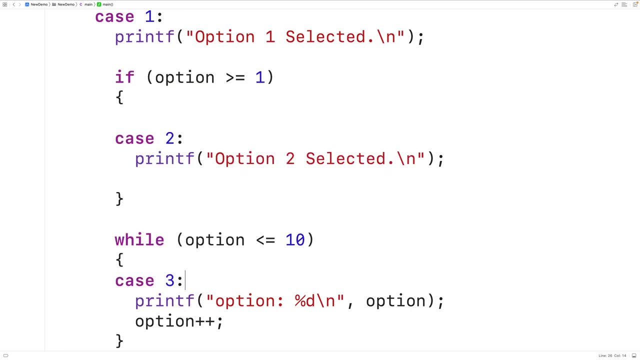 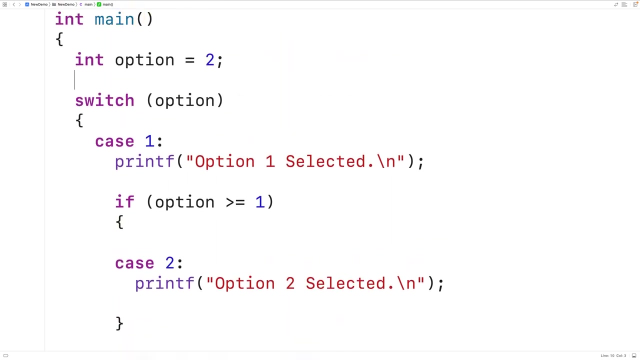 iteration And we'll also output option 2.. So we'll have printf option, colon percent d, backslash n to print And then option inside this loop body. we'll have case 3, and this is also valid. We can have a case right in the middle of a loop. So for example, if we change option to 3 here now, 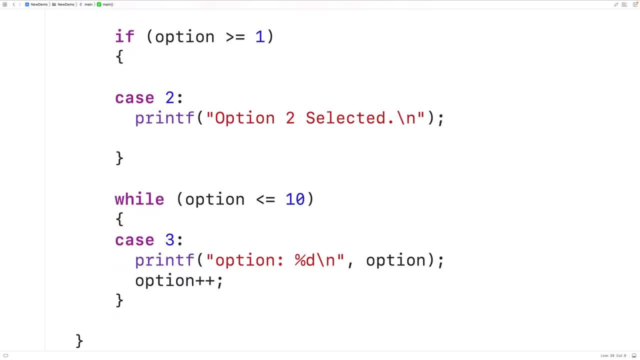 and then we save, compile and run the program, execution is going to jump down to case 3.. If we save and compile and run the program, we're going to see that we get option 3, option 4, down to option 2..